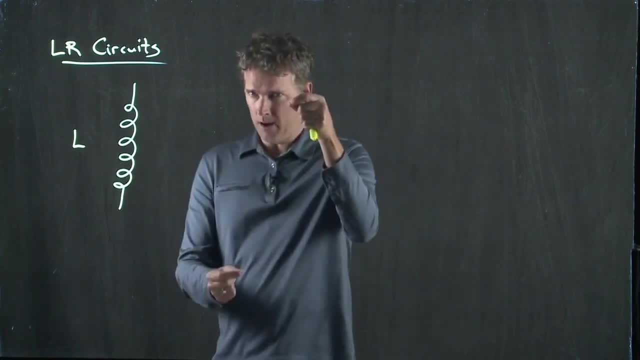 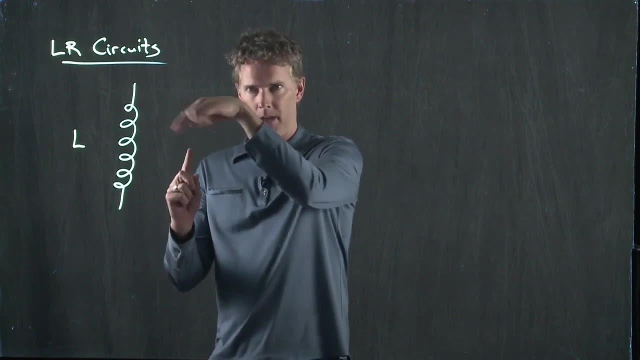 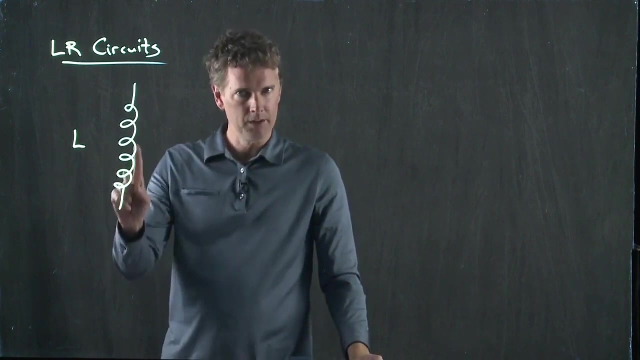 an inductor, which is kind of weird, right, Because the wire, when it's straight, behaves very differently than the same wire that's just coiled up in this spring. And the difference, of course, is this one has magnetic field propagating through the center of it, The 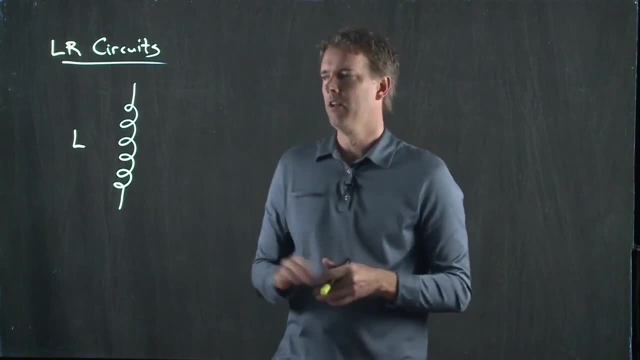 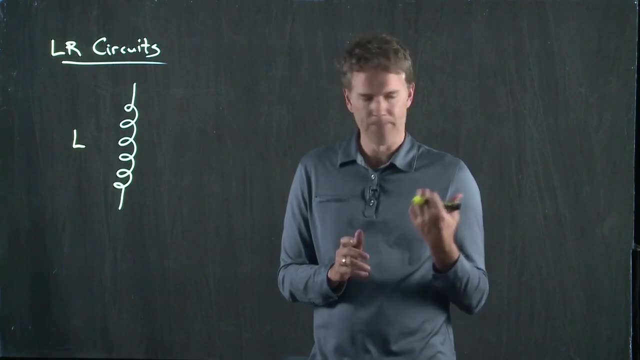 straight wire doesn't have magnetic field propagating to the center of it, So this device, the inductor, behaves interestingly, very different than a wire. Okay, let's talk about what this looks like in a circuit. So let's say we do the following. Let's take 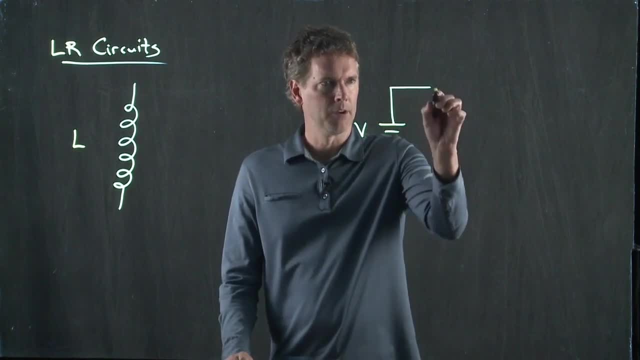 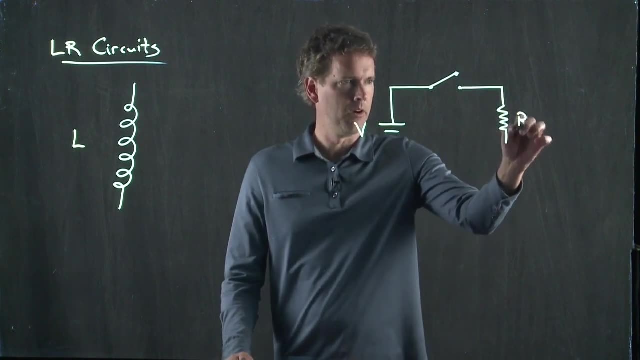 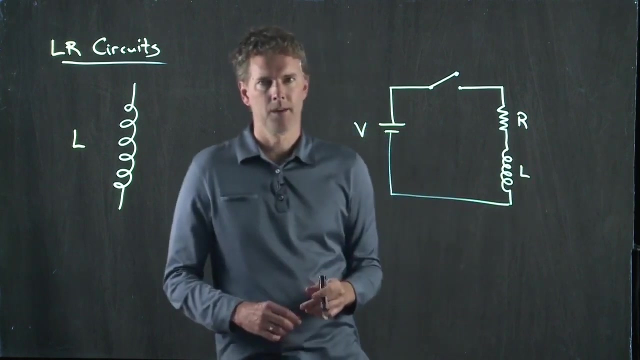 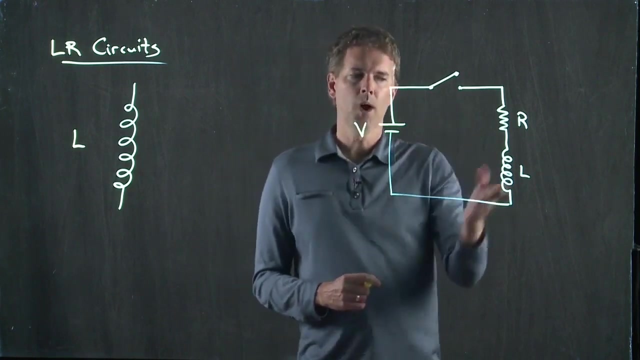 a battery voltage V, and let's hook up a switch to the battery. And now we will put a resistor R and an inductor L, Okay, And all we're going to do is close the switch. And if we close the switch, what happens to the current in the circuit? And how do we? 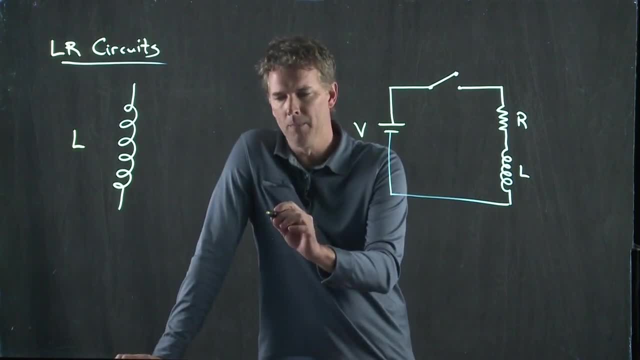 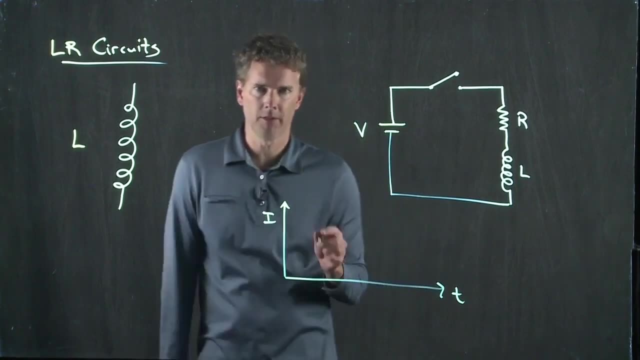 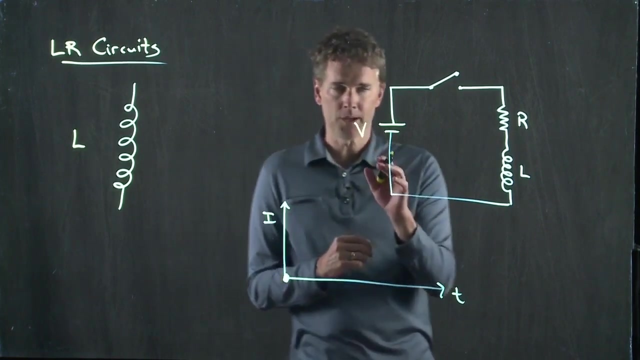 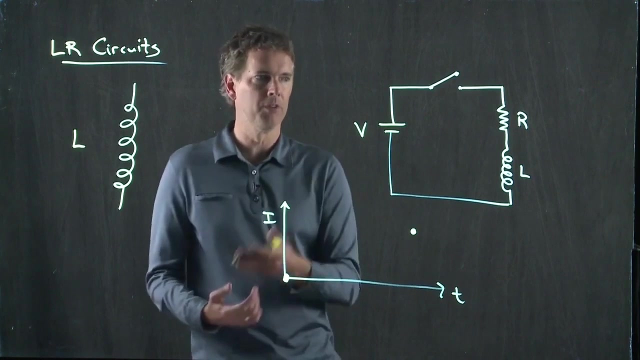 figure this out. What we figured out is we go back to our limits. If I think about the current in the circuit as a function of time before the switch is open, it's obviously zero. After the switch is open for a long time, there should be some sort of steady state current that goes through. 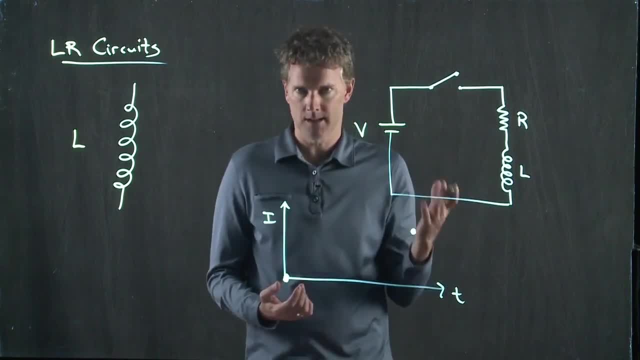 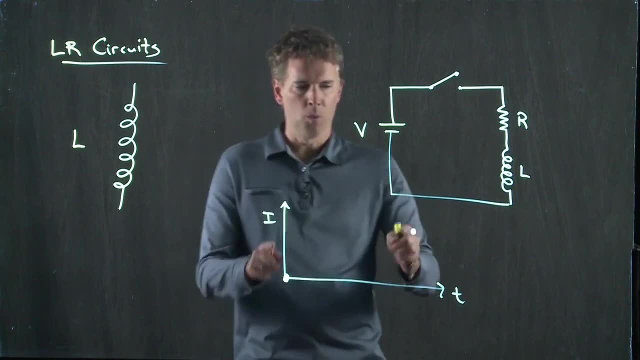 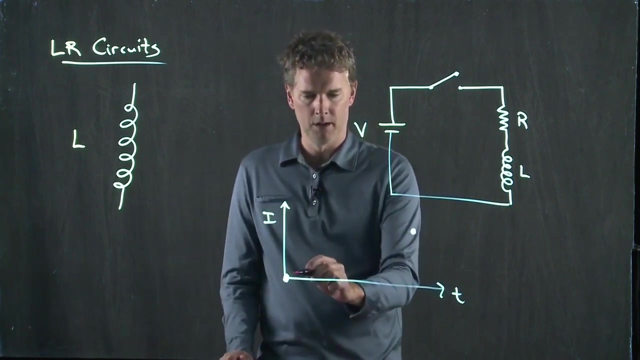 the circuit Okay, And it shouldn't be changing in time anymore. It should just be some steady state value. So, just like we talked about with capacitors, when we have two points and we want to connect them, we have a bunch of different options. One option: is this a straight line Okay? 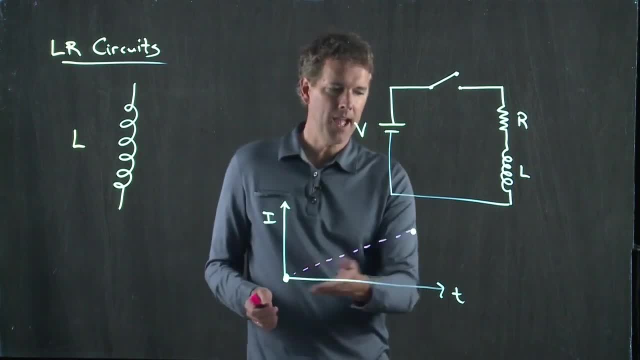 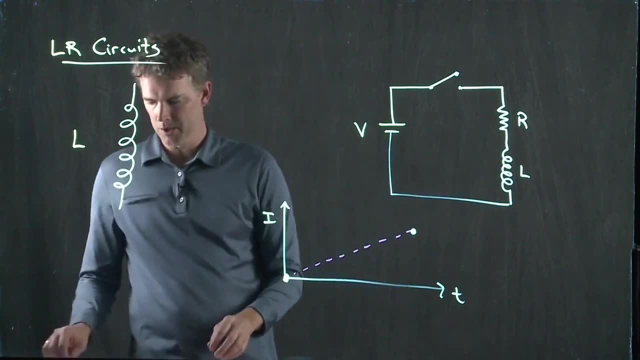 But a straight line doesn't make a lot of sense because as time goes on, it says that current would just keep going up and up and up. So we don't like that one very much. Okay, So we're going to erase that one. 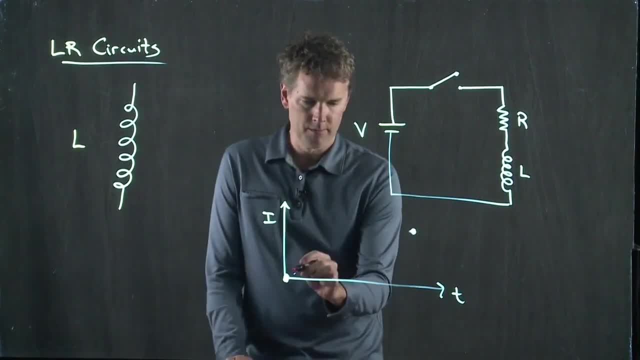 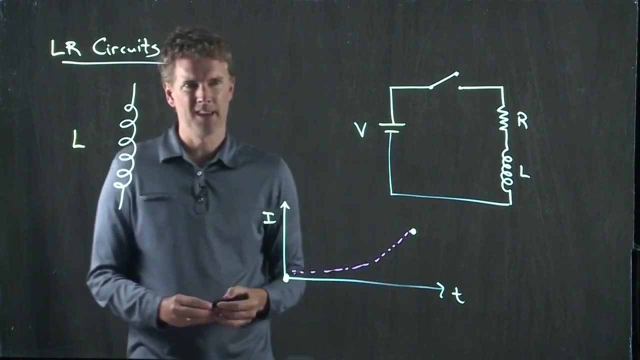 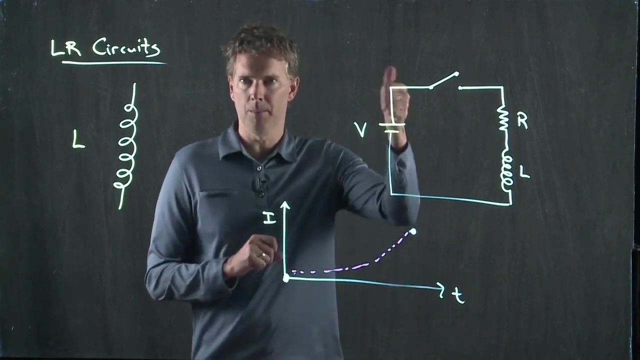 What about? What about? What about a curve that goes like this? We don't like that one very much either because, again, as time goes on, it says the current should just keep going up and up and up. But we know that can't be the case, right, Ultimately. 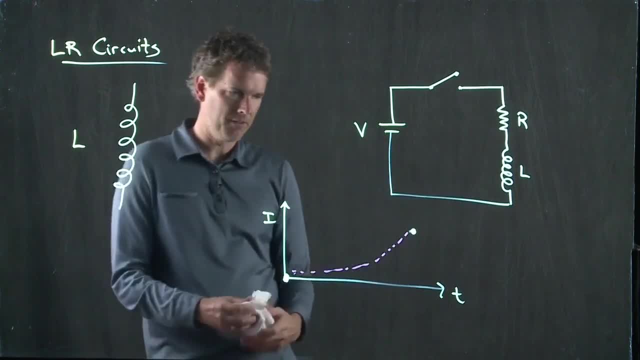 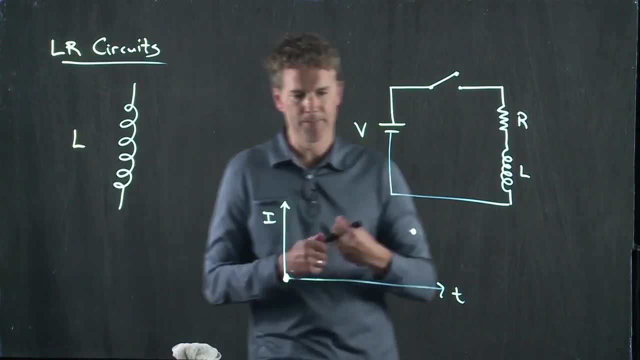 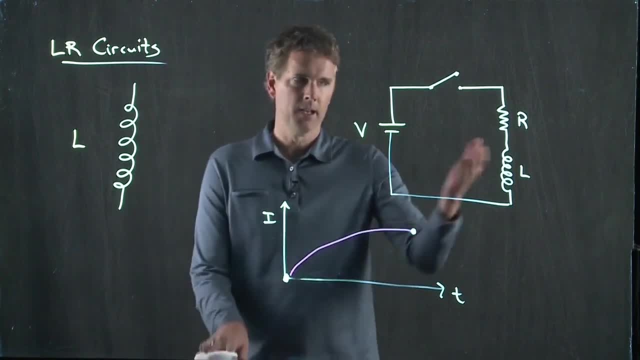 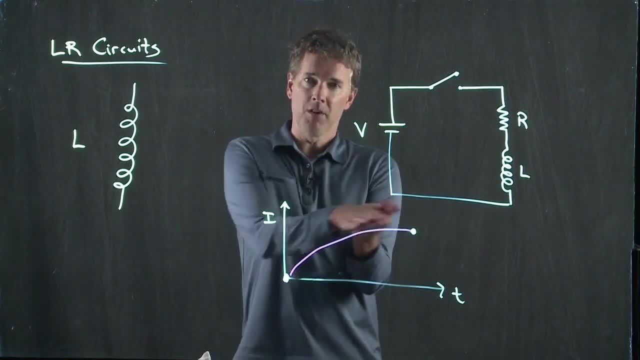 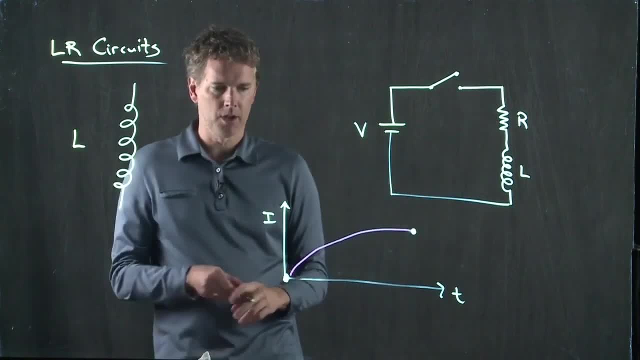 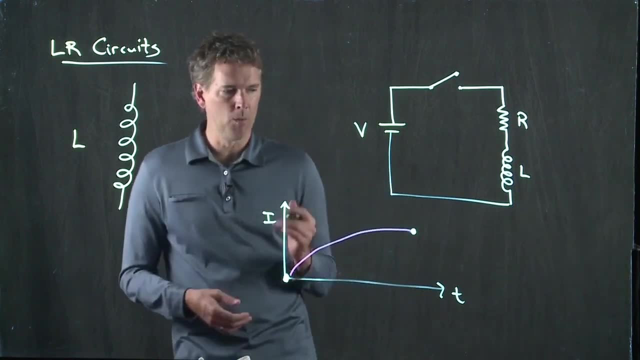 We have a point here. We have a point here: The resistor is ultimately going to limit how much current can go through the system, and this is a curve that you end up with. And now you can probably map out what this is going to look like. 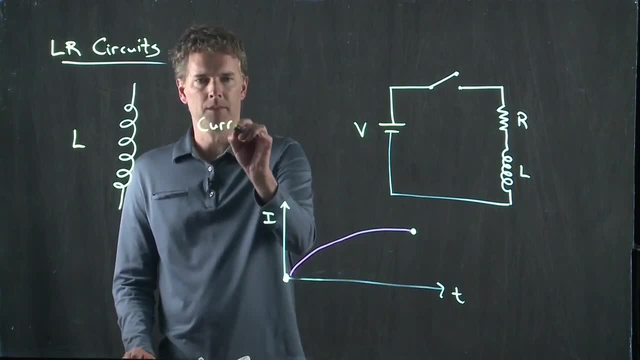 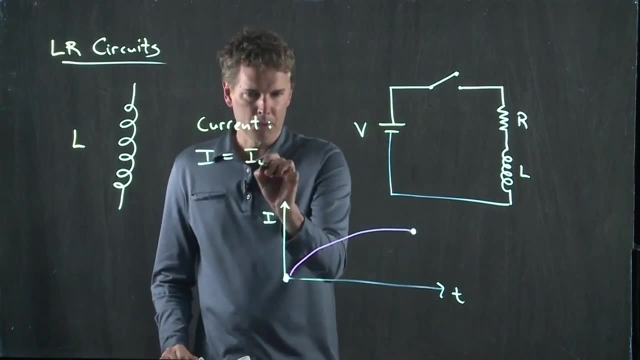 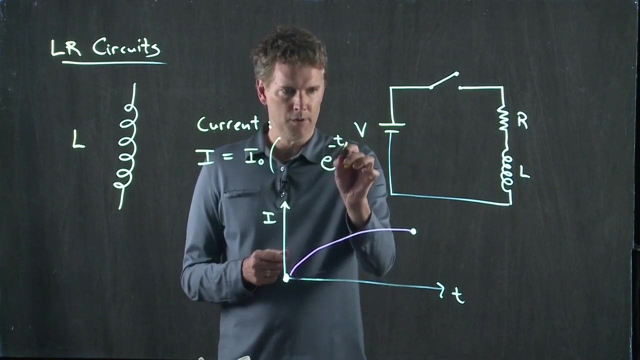 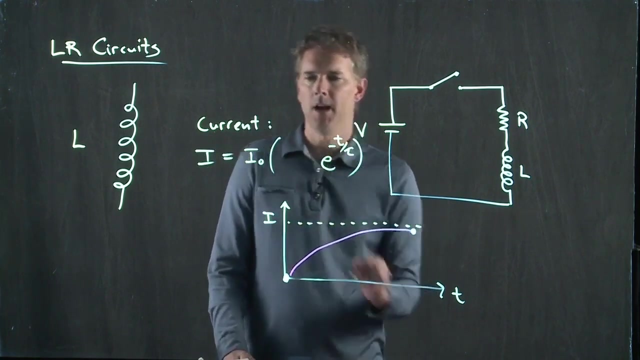 Just like we did with the capacitors. the current is going to behave like an exponential. There is some maximum current that it can have- I0. We know that there is an e to the minus t over tau i's somewhere. and now, if we're going to get up to this level of I-naught, we have to put. 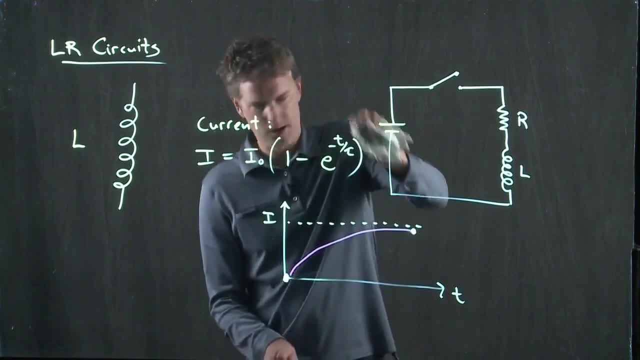 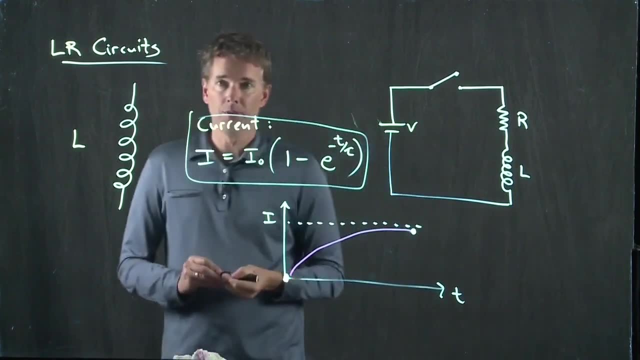 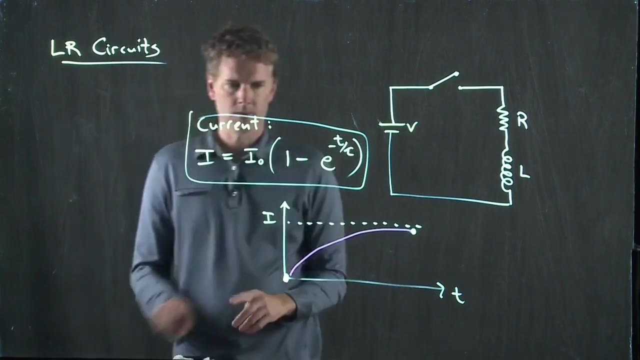 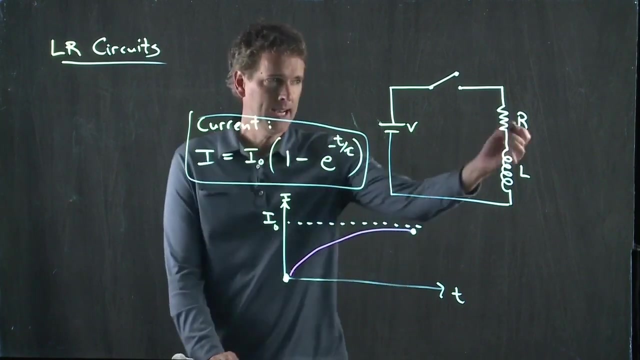 a one minus. Let's move this V so we're not confused with that one. This is what the current looks like in this system. What are the different values in this function? I-naught is just the maximum current. That's where you end up, right there. That has to be related to. the resistor, because after a long time where the current is steady, the inductor doesn't do anything anymore. It's just going to act like a wire. Remember, inductors only are resisting changes in current, so eventually it's just going to look like a wire. So I-naught. 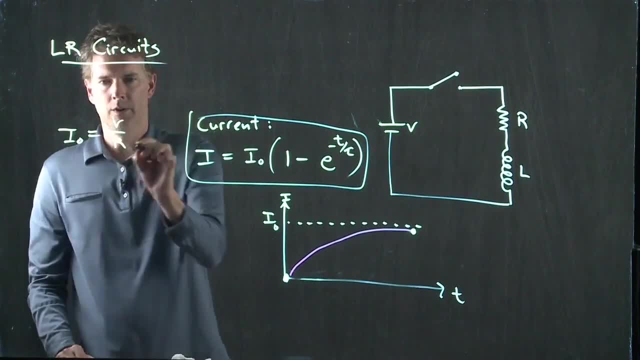 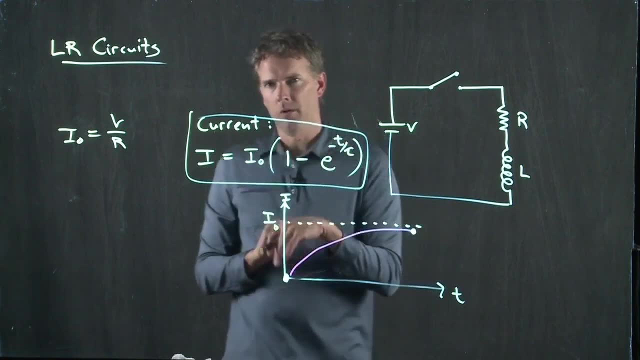 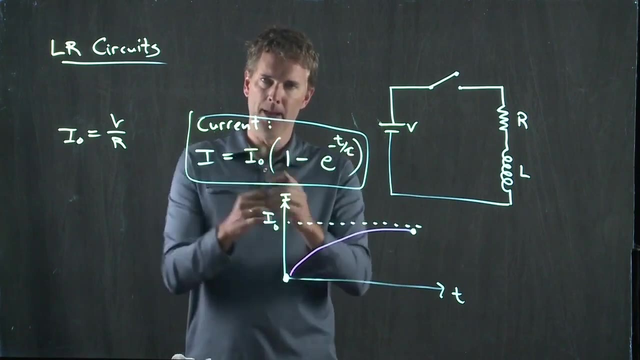 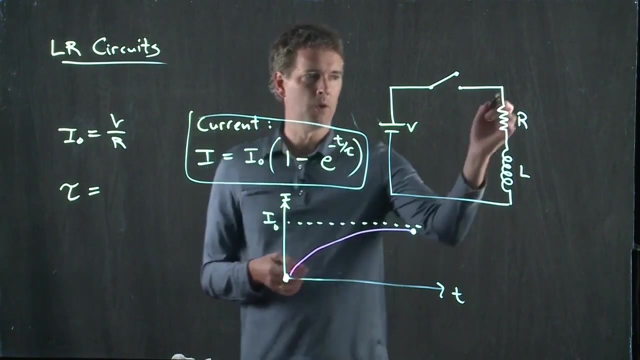 is just going to be V over R. Good old Ohm's Law. What about tau? Remember, before for tau we had a time constant that went like RC, when we had a big capacitor, longer time constant, Big resistor, longer time constant. So tau here has got to be related to R and to L. but we need to make sense of 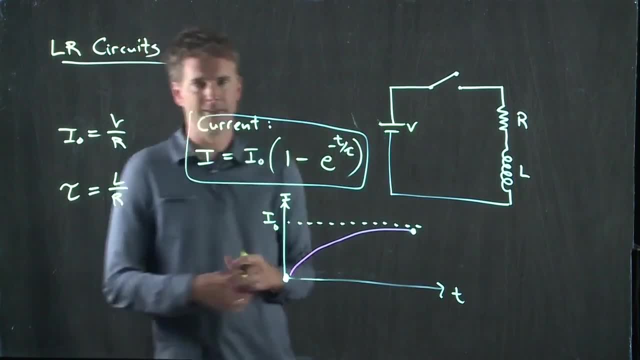 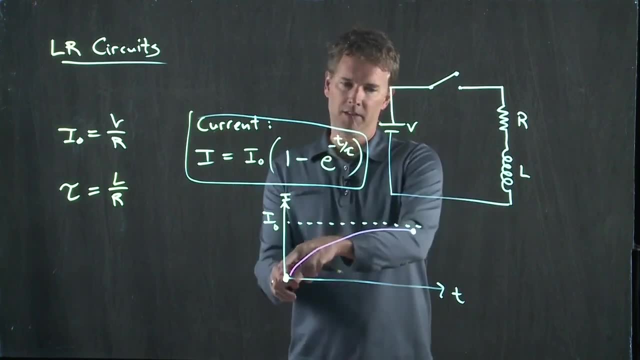 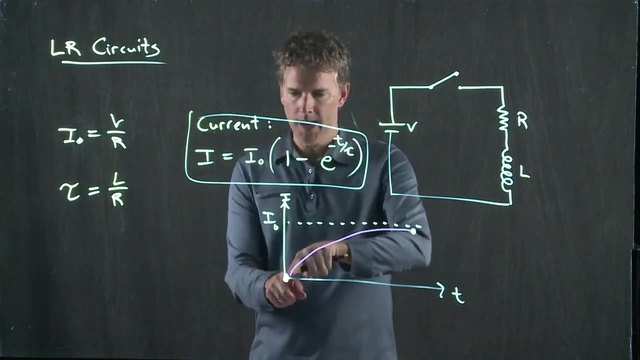 which way it should be. So tau is equal to L-naught divided by R. okay, If I have a very big inductor, that time constant gets very long. This thing stretches out quite a bit. If I have a very big resistor, the time constant gets short and it. 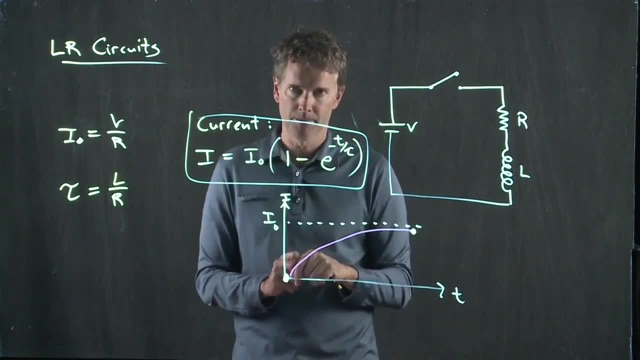 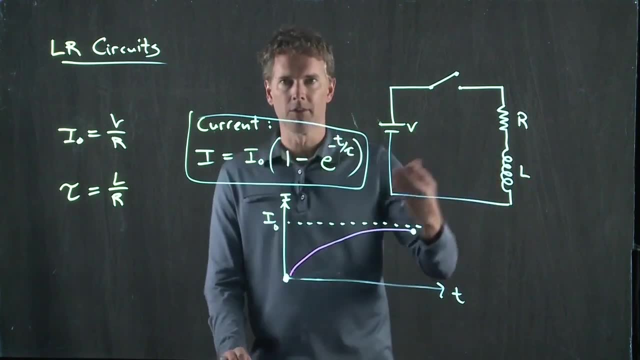 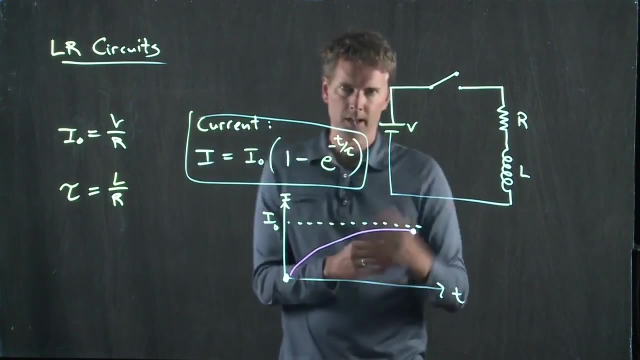 quickly goes up to the maximum value. okay, And that's because, ultimately, not much current is going to flow in the system, and so the inductor is less concerned about the changing current. all right, So this is the equation for the current in an LR circuit, like we showed here. 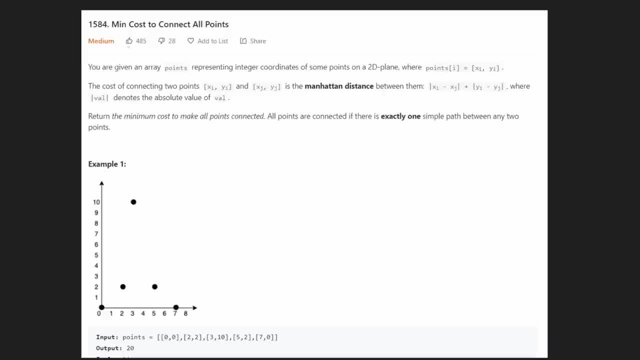 Hey everyone, welcome back and let's write some more neat code today. So today let's solve minimum cost to connect all points And, surprise, this actually is not a problem from the blind 75 list that we've been working on recently And the reason I'm solving this problem is because, honestly, 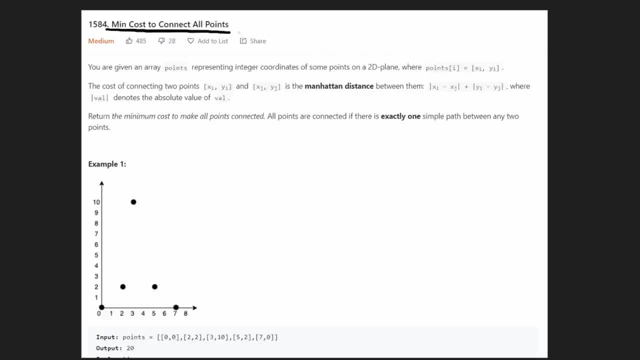 it actually should be a part of that list, Like this is one of those problems. I think that's missing from the blind 75 list. Reason being is: this is a problem related to minimum spanning trees, a concept that a lot of people skip over, I think, when they grind leak code. So this is. 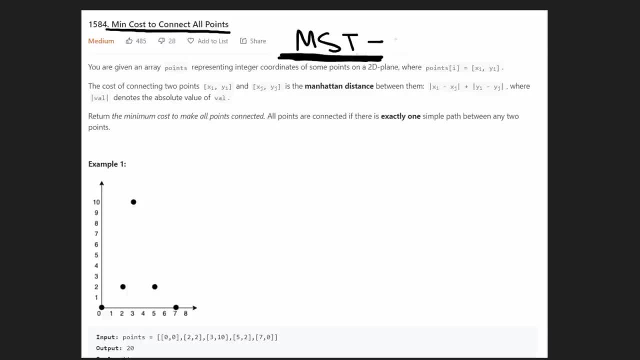 what we're going to be doing today, And you might have heard of an algorithm for minimum spanning trees. There's actually a couple Prim's algorithm and there's also Kruskal's. We're going to be doing Prim's algorithm because I think it's easier to implement and it's actually more efficient most. 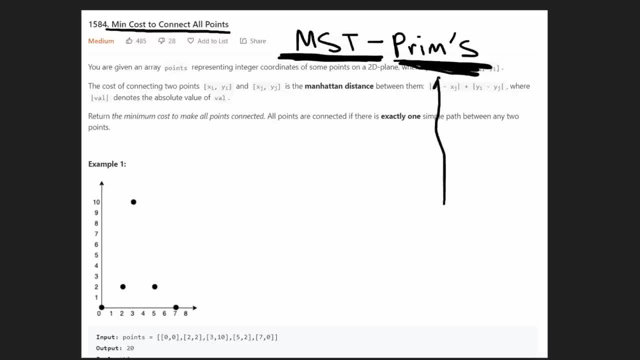 of the time, And you might remember this algorithm from college. Most computer science curriculums do teach it, but if you're anything like me, you probably forgot it the instant that you finished the class that you learned it in. But that's okay, And this algorithm Prim's. 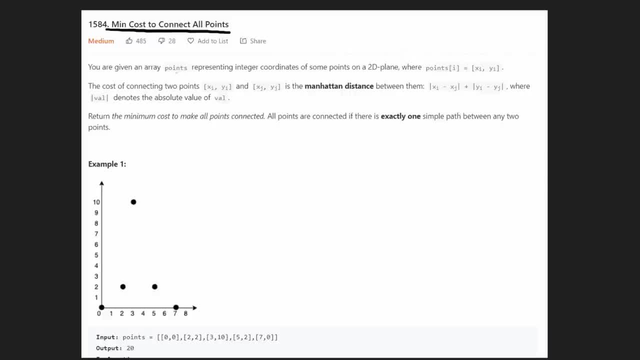 algorithm is actually not as complicated as you might expect. So we're just given a list of points that represent some coordinates on a 2D plane. So for each point we're given two values: the x-coordinate and the y-coordinate. So the cost of connecting any two particular points, like let's